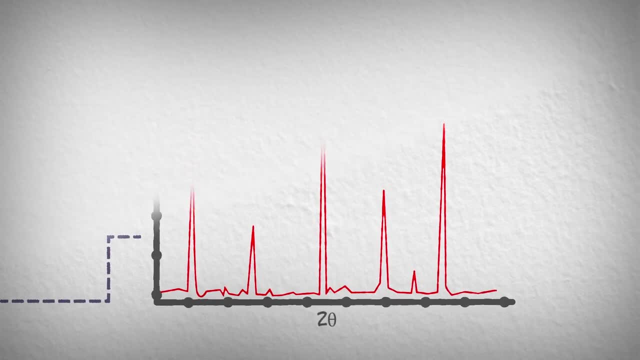 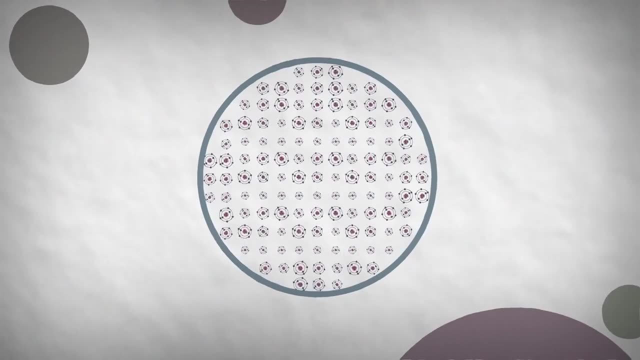 where peaks are observed, related to the atomic structure of the sample. Most materials are made up of many small crystals, like sand on a beach. Each of these crystals is composed of a regular arrangement of atoms, and each atom is composed of a nucleus surrounded by a cloud of electrons. 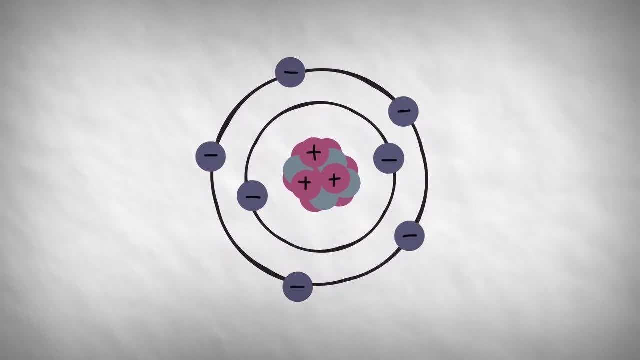 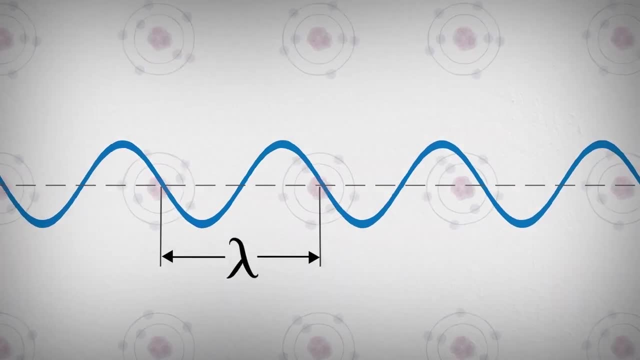 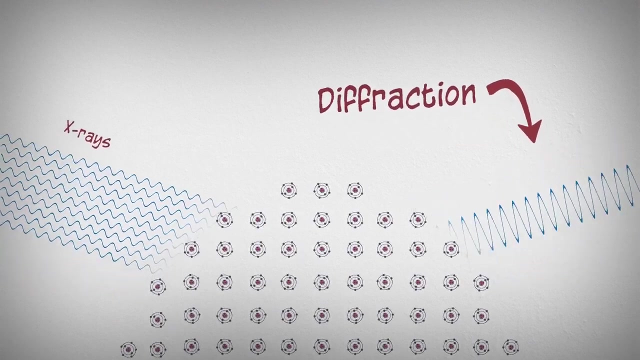 It's at this scale that the story of x-ray diffraction begins. X-rays are high-energy light with a repeating period called the wavelength. Since the wavelength of an x-ray is similar to the distance between atoms in a crystal, a special interference effect called diffraction can be used to measure the distance between atoms. 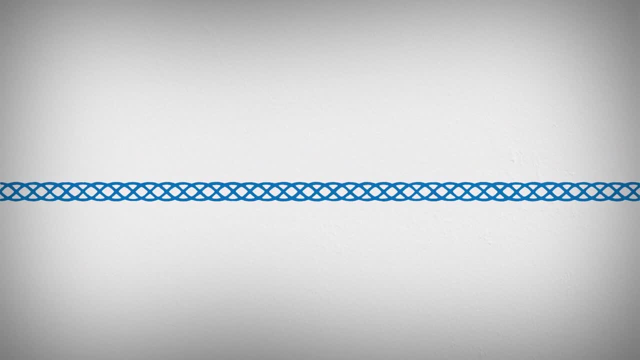 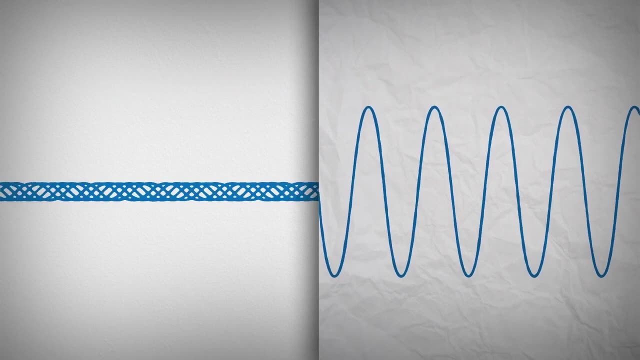 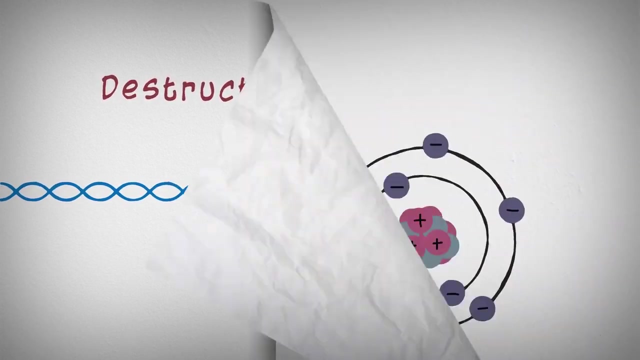 Interference occurs when x-rays interact with each other. If the waves are in alignment, the signal is amplified. This is called constructive interference. If the waves are out of alignment, the signal is destroyed. This is called destructive interference. When an x-ray encounters an atom, its energy is absorbed by the electrons. 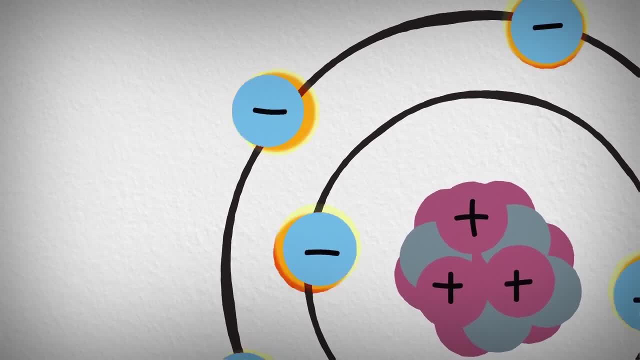 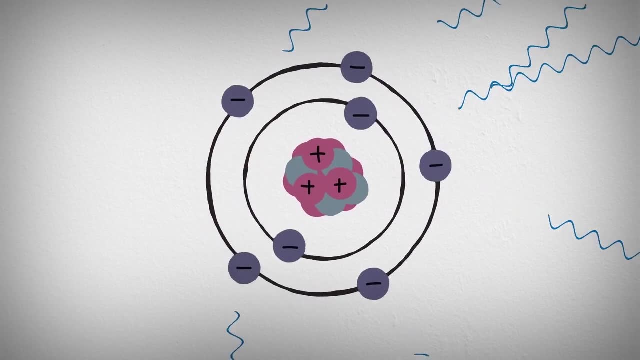 Electrons occupy special energy states around an atom. Since this is not enough energy for the electron to be released, the energy must be released. The electron's energy must be re-emitted in the form of a new x-ray with the same energy as the original. 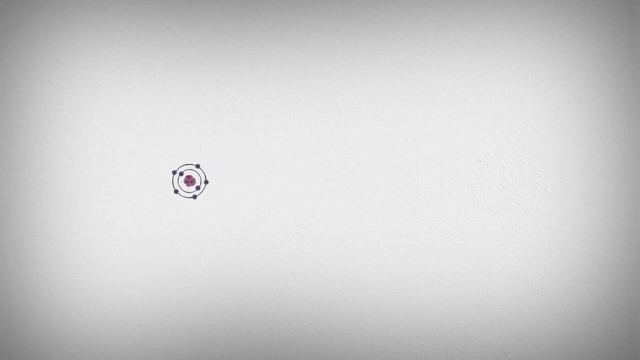 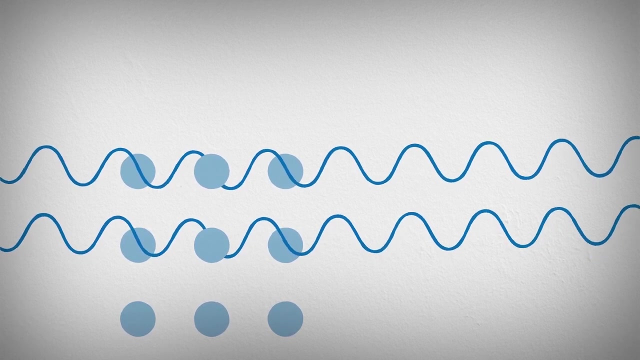 This process is called elastic scattering. In a crystal, the repeating arrangement of atoms form distinct planes separated by well-defined distances. When the atomic planes are exposed to an x-ray beam, x-rays are scattered by the regularly spaced atoms. Strong amplification of the emitted signal occurs at very specific angles. 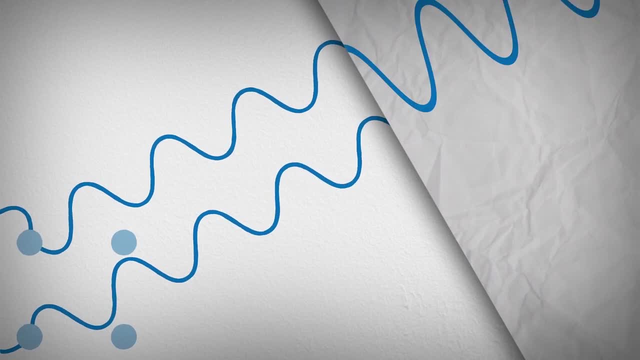 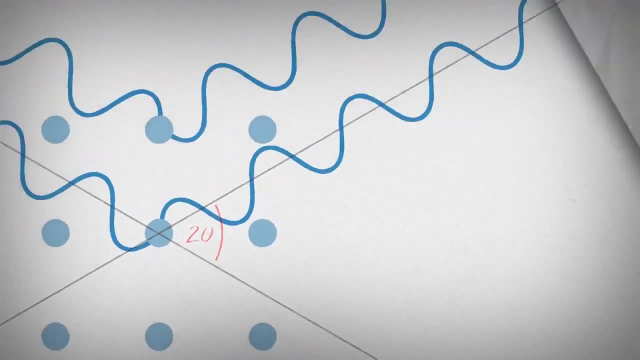 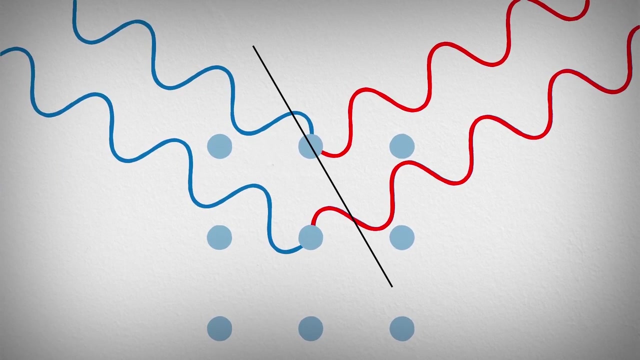 where the scattered waves constructively interfere. This effect is called diffraction. The angle between the incident and the scattered beam is called 2-theta. In order for constructive interference to occur, the scattered waves must be in alignment, meaning that the second wave must travel a whole number of wavelengths. 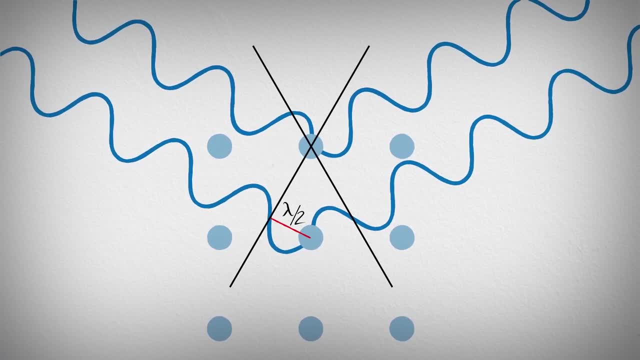 In this case, one-half of a wavelength is traveled on the incident side and one-half on the scattered side, yielding one additional wavelength. In the case of the next x-ray, one wavelength is traveled on both the incident and the scattered side, resulting in two wavelengths. 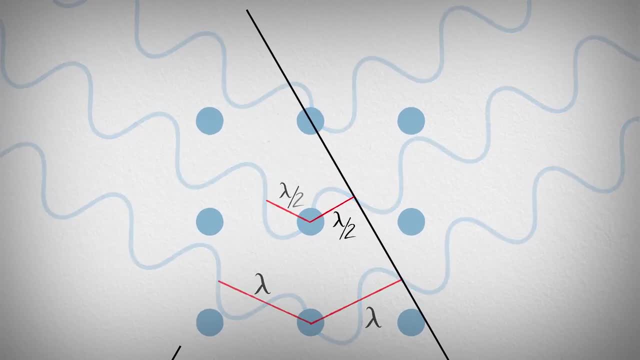 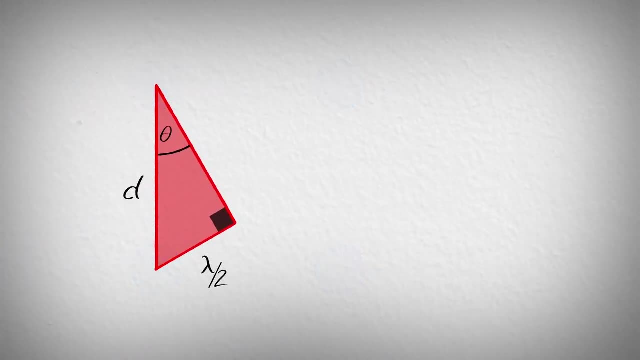 This reinforcement occurs throughout the crystal. The exact angle at which diffraction occurs can be determined from the red triangle. The angle at the top is theta half the angle between the incident and scattered beams. The long side is the distance between the atomic planes.